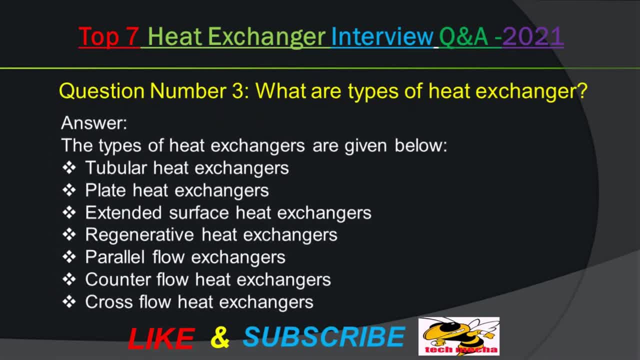 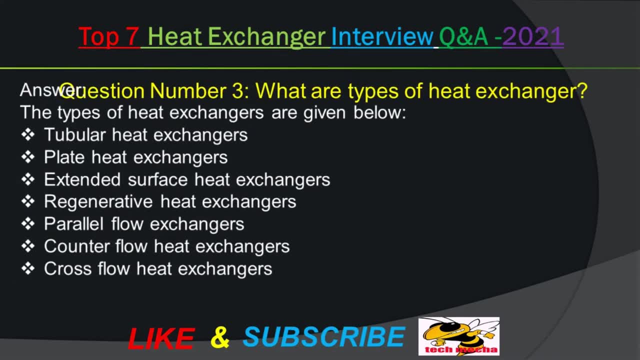 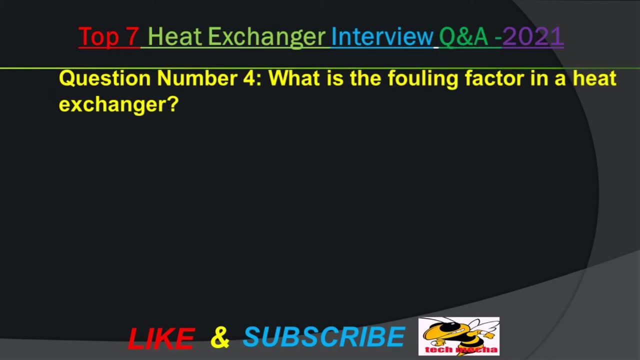 extended surface heat exchangers. regenerative heat exchangers, parallel flow exchanges, counter flow heat exchangers, cross flow heat exchangers. question number four: what is the fouling factor in a heat exchanger? answer: fouling is a general term that includes any kind of deposits of extraneous material that appears on the heat. 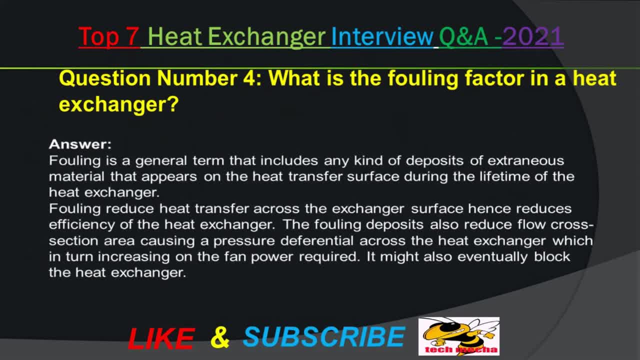 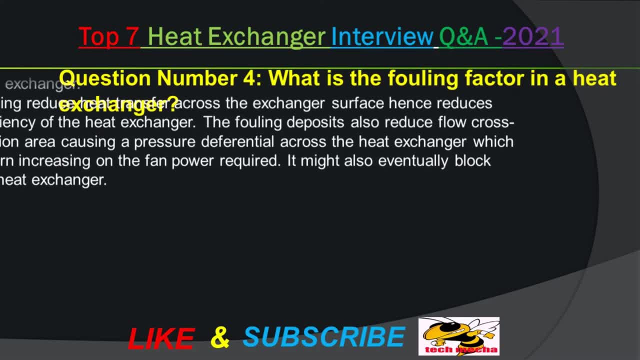 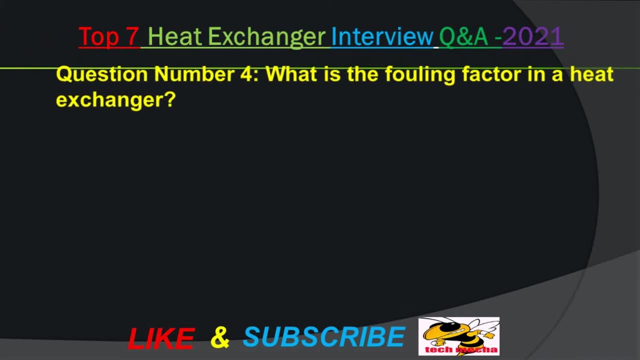 transfer surface during the lifetime of the heat exchanger. fouling reduce heat transfer across the exchanger surface, hence reduces efficiency of the heat exchanger. the fouling deposits also reduce flow cross-section area, causing a pressure differential across the heat exchanger which in turn increasing on the 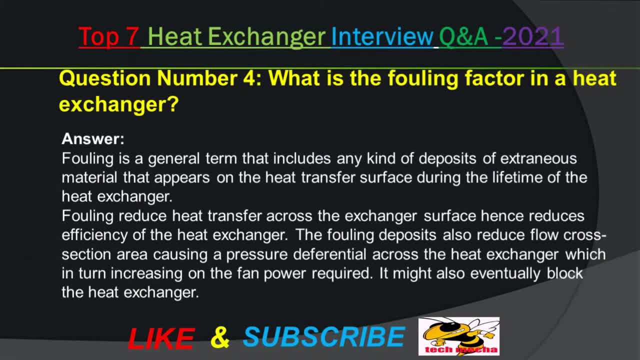 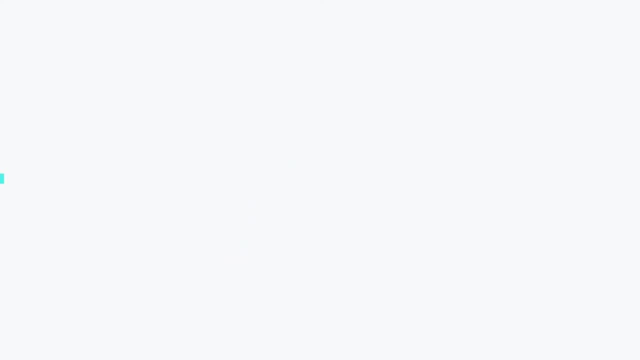 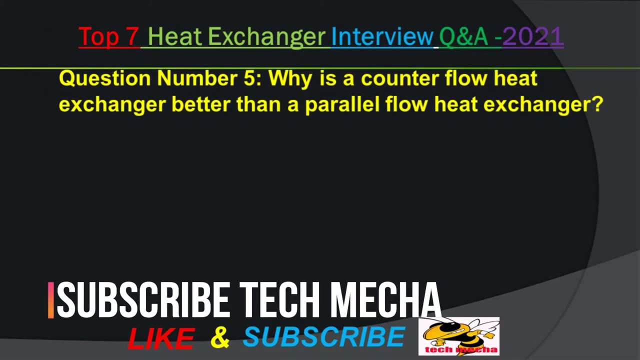 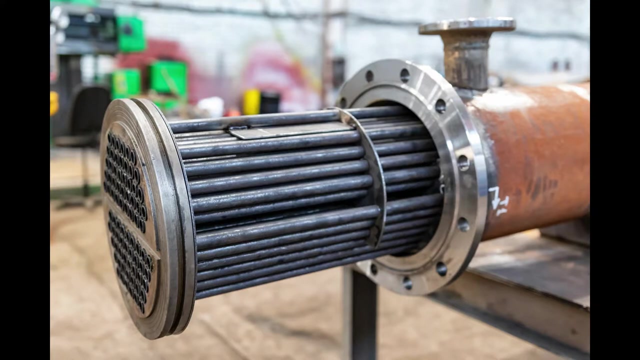 fan power required, it might also eventually block the heat exchanger. question number five: why is a counter flow heat exchanger better than a parallel flow heat exchanger? answer: in counter flow arrangement the temperature difference between the hot fluid and cold fluids is fairly constant across the heat exchanger, he which enhances the rate of heat. 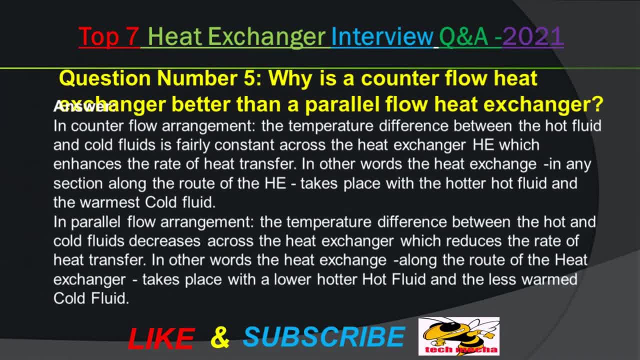 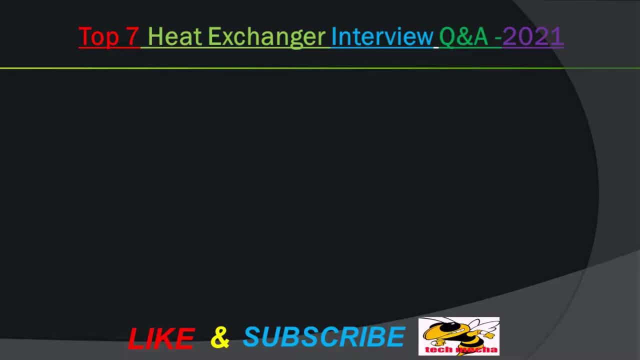 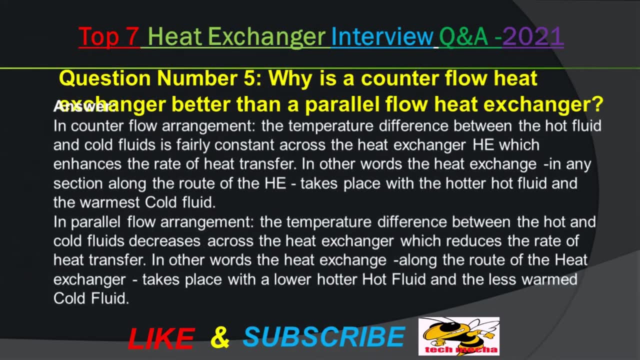 transfer, in other words the heat exchange in any section along the route of the. he takes place with a hotter hot fluid in the warmest cold fluid. in parallel flow arrangement, the temperature difference between the hot and cold fluids decreases across the heat exchanger, which reduces the rate of heat transfer, in other words, the heat exchange along the route of the heat. 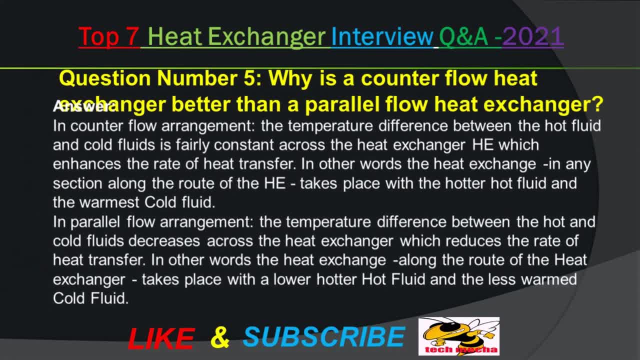 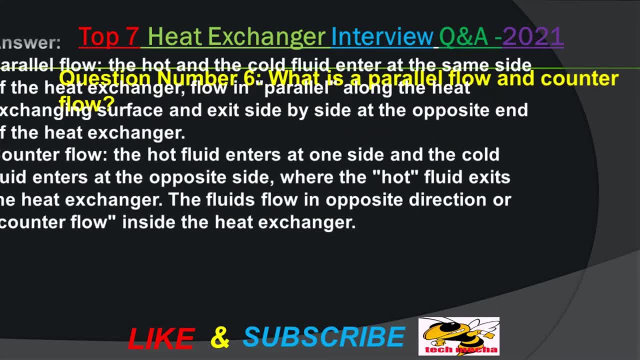 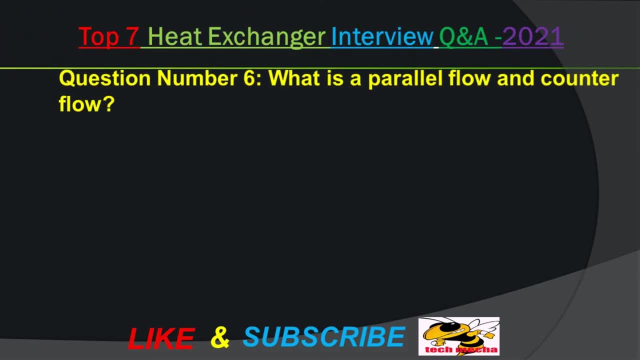 exchanger takes place with a lower hotter hot fluid in the less warmed cold fluid. question number six: what is a parallel flow and counter flow? answer: parallel flow: the hot and the cold fluid enter at the same inside the heat exchanger, flowing parallel along the heat exchanging surface. 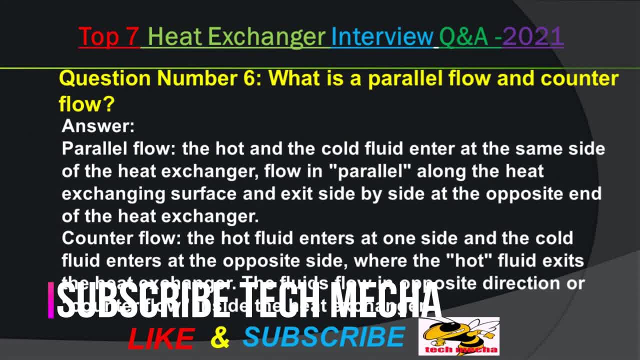 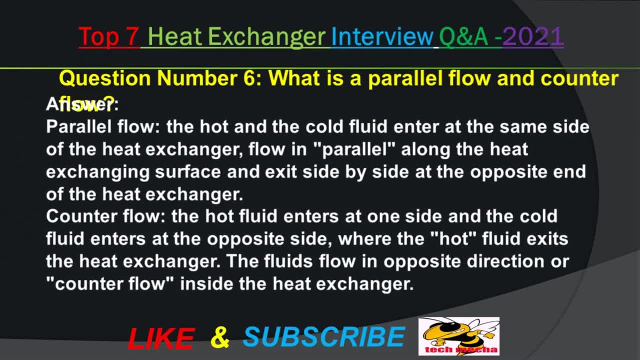 and exit side by side. at the opposite end of the heat exchanger- counter flow- the hot fluid enters at one side in the cold fluid enters at the opposite side. where the hot fluid exits the heat exchanger, the fluids flow in opposite direction or counter flow inside the heat.